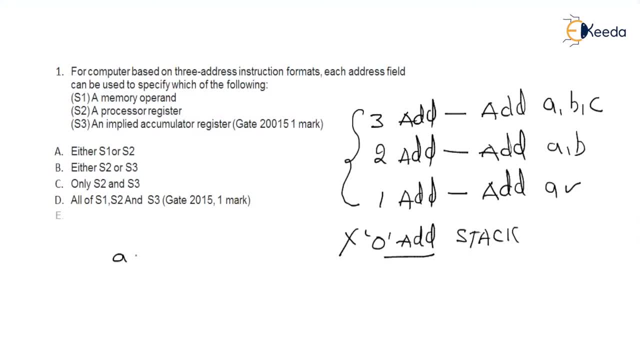 are going to execute it. You know that in one address instruction add a. when it is getting executed it will lead to an operation. Accumulator is equal to accumulator plus a, The value of memory location. a gets added to accumulator and finally will get transferred. 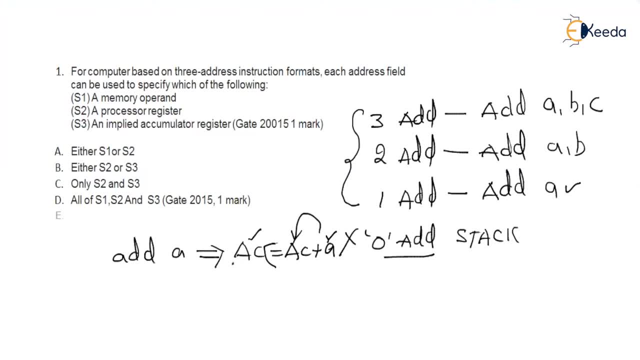 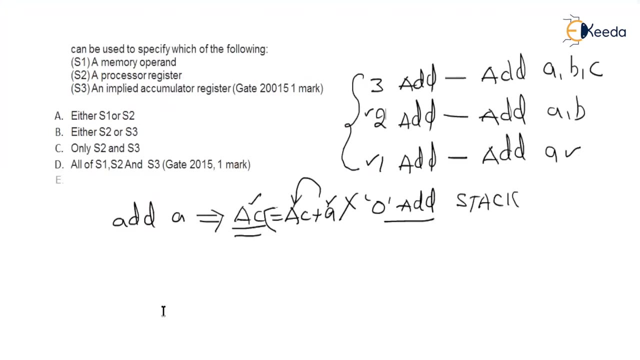 to accumulator, Right? So accumulator is an implicit and an implied operand in only one address instructions. But when it comes to two address, let us have a look at how these instructions are going to get executed In two address. the instruction may be like: add a- b, which will lead to an operation that is: a is equal. 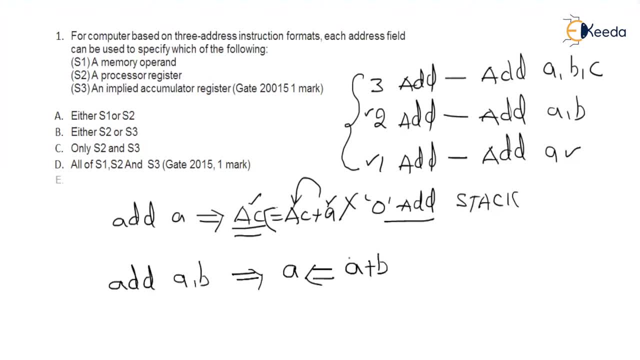 to a plus b Memory location. sorry, the contents of the memory location a will get added to the contents of the memory location b will get transferred to a. So a is a source as well as the destination and b is just a source operand. Okay. 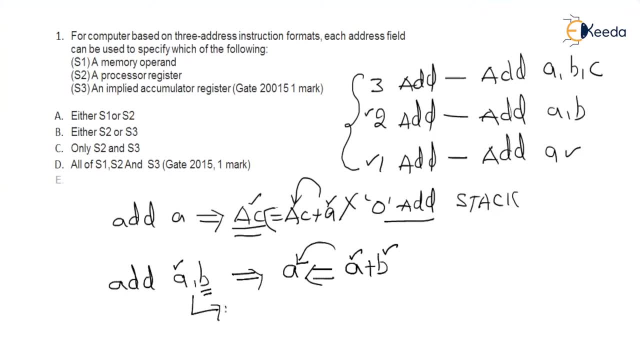 These two operands could be either a memory location or a register in the processor. Okay, That is. you can also see an instruction such as r1, r2.. So this is add a, b and which is going to perform an operation in between two memory operands. 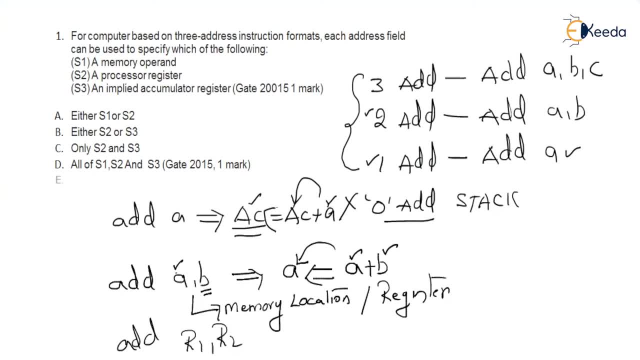 And, finally, value will get transferred to a memory operand. The same thing if it is being performed in between two processors register: the value will get added and finally gets transferred to a processor's register. Similarly, when it comes to three-address instruction. 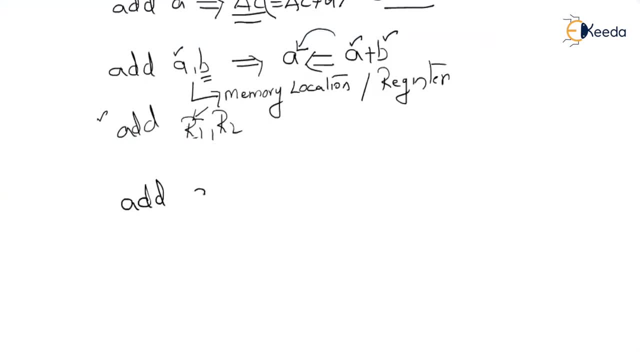 it will look like: add, a, b, c, in which the operation is a is equal to b plus c. Okay thing is, these three operands can be either a processor's register or a memory location, such as R1, R2, R3.. So in these positions in the instruction, first operand and second.